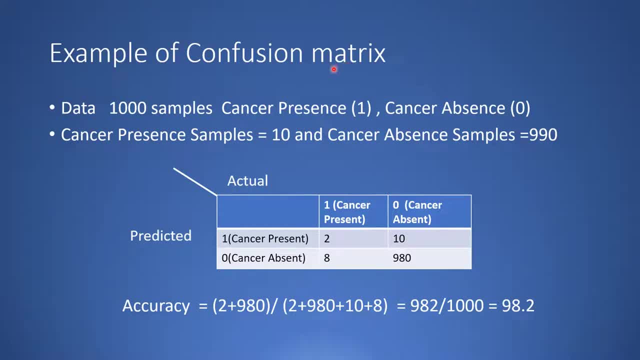 Let us look at an example of a confusion matrix. So here we have 1000 samples in our data and the positive class is cancer presence and the negative class is cancer absence. Right, So we have 10 positive samples and we have 990 negative samples. Okay, So we have, we have a machine learning algorithm which is trained to detect whether cancer is present or not. Okay, So now we ran that algorithm on this machine learning algorithm. 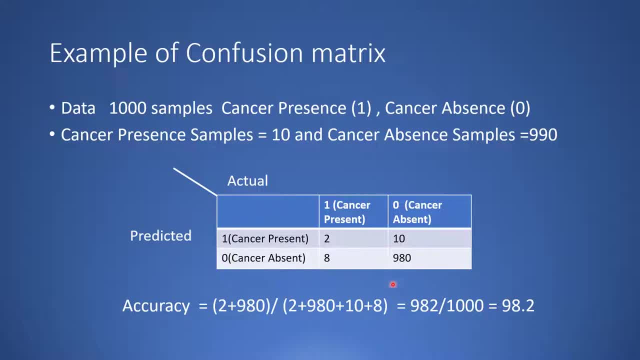 This data set Okay, And we get this kind of a confusion matrix Okay. So again, you have the actual classes, You have the predicted classes, You have the positive and the negative classes. So if you look over here, out of 10 you know samples which have cancer. only 2 are predicted as having cancer, 8 is being predicted as cancer is absent, Right, And out of 990 samples where cancer is present, 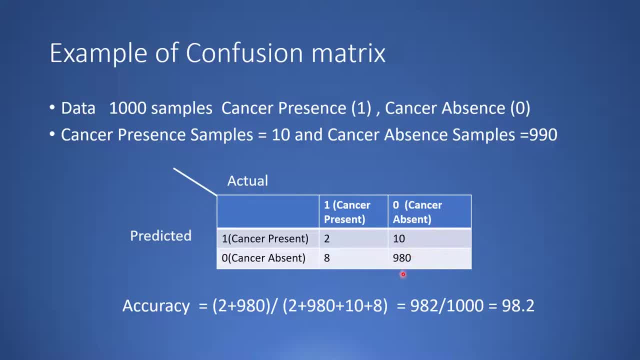 It is actually predicting 980 samples as cancer is absent and 10 samples as cancer is present. Okay, So this is your true positive, This is your true negative. This is your false positive and this is your false negative. Now, if you do the accuracy computation over here, you see that the accuracy comes close to 98.2%. Right Now, this is very good accuracy, Right, But what is the accuracy? 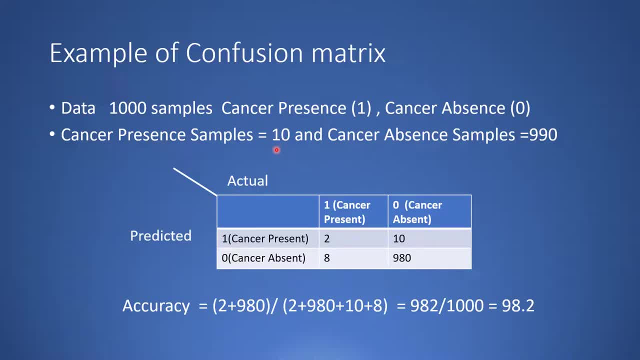 This is the flaw over here. This is a kind of an imbalanced data set. Right, The number of positive classes is very small. Okay, You can even invert it and say that this is a positive class, which is cancer absence and cancer presence is the minority class. Right, It is the negative class. Even then, it's an imbalanced data set. So in case of an imbalanced data set, the accuracy is not a good measure because if you look at this algorithm, we are missing. 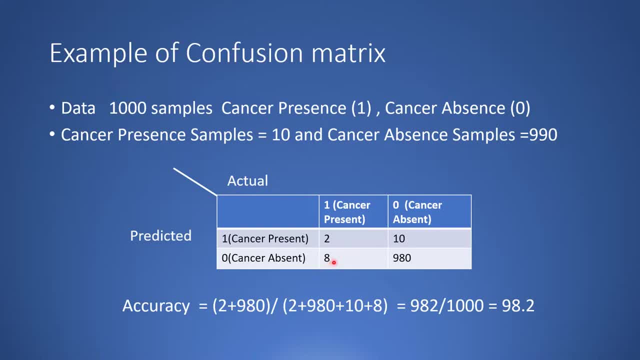 8 cancer patients over here who have cancer, but they are getting predicted as they don't have cancer right. so this is actually a limitation of looking at accuracy as a metric for the performance of classification algorithms.